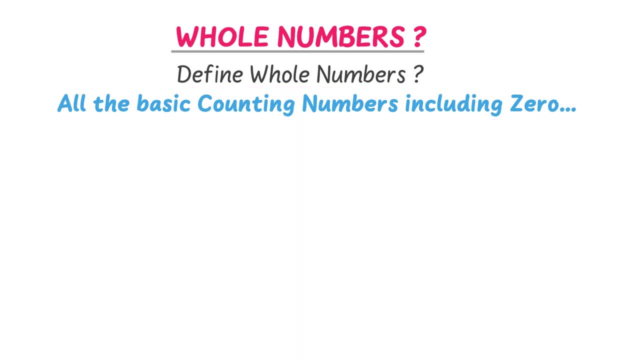 including zero, are called whole numbers. The set of whole numbers is denoted by W, And it contains all numbers like 0,, 1,, 2,, 3,, 4 and so on. Whole numbers include natural numbers that begin from 1.. Secondly, whole numbers also include all. 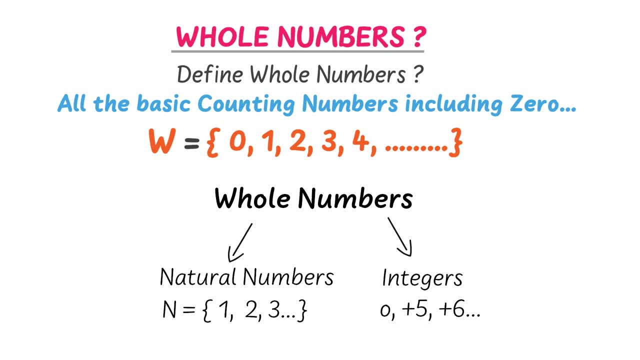 positive numbers. So if you have a set of whole numbers, you can use all these numbers. You can use positive numbers to count all the positive integers along with zero. Thirdly, all the positive numbers on a number line are whole numbers like 0,, 5 and 6.. Thus, 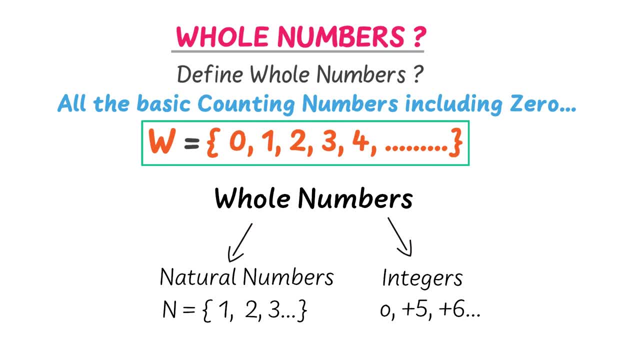 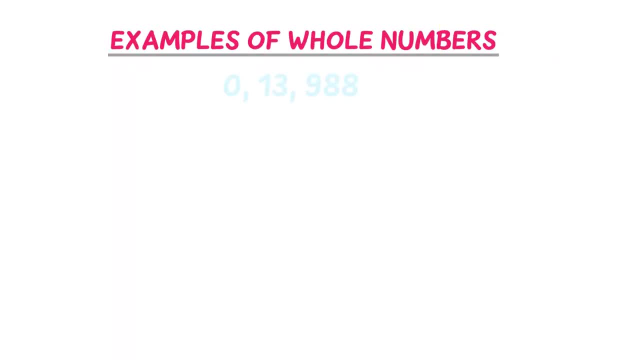 remember that all the numbers which we use for counting purposes, including zero, are whole numbers. Now let me teach you some examples of whole numbers. Zero is a whole number. Thirteen is a whole number. Nine hundred eighty-eight, also a whole number, No, what are not whole numbers? Well, all the negative numbers are. 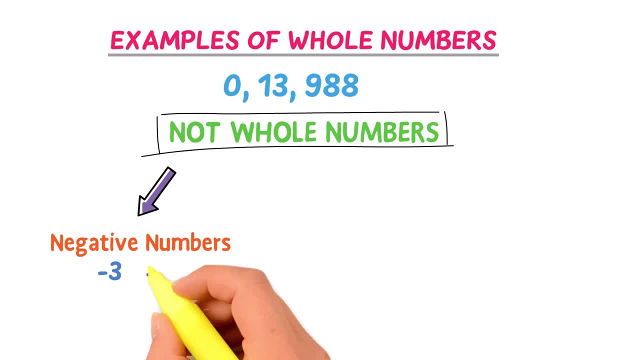 not whole numbers, like minus 3, minus 20, etc. Secondly, all the decimal numbers are not whole numbers, like 3.6, 8.9, etc. Thirdly, all the numbers in friction or p by q form are not whole numbers, like 2 upon 3, 1 upon 6, etc. Finally, let me teach you some important 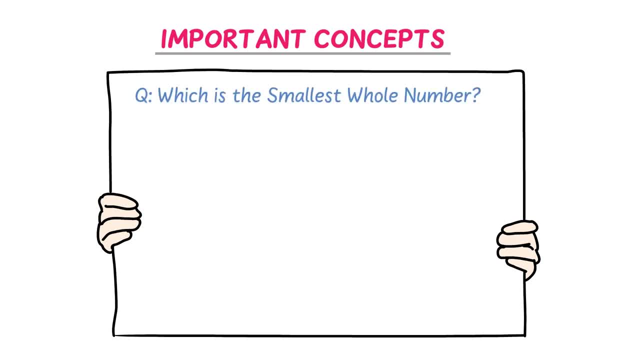 concepts of whole numbers like: which is the smallest whole number? Well, 0 is the smallest whole number. There is no predecessor or a number that comes before 0.. Let me repeat this important statement: There is no predecessor or a number that comes. 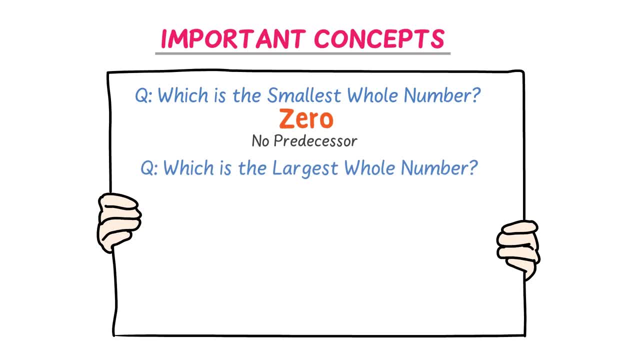 before 0.. Let me repeat this important statement: There is no predecessor or a number that comes before zero. Secondly, which is the largest whole number? Remember that there is no largest whole number, or we can say that no number is considered to be the largest whole number. Thirdly, can whole? 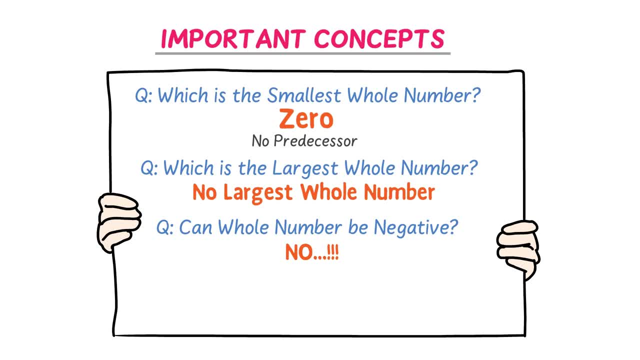 numbers be negative? Well, the answer is no. Whole numbers cannot be negative. Fourthly, can natural numbers be considered as whole numbers? The answer is yes, All the natural numbers are also considered as whole numbers, But not all the whole numbers are considered as the natural numbers. To summarize, 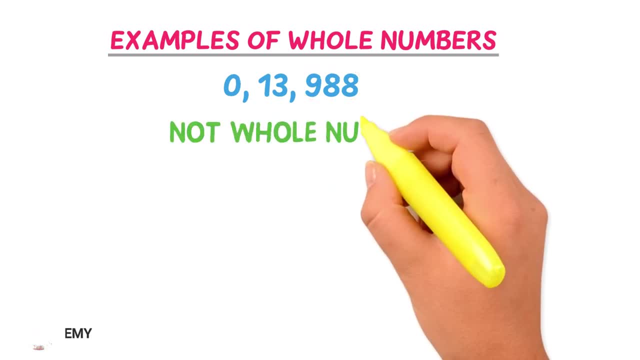 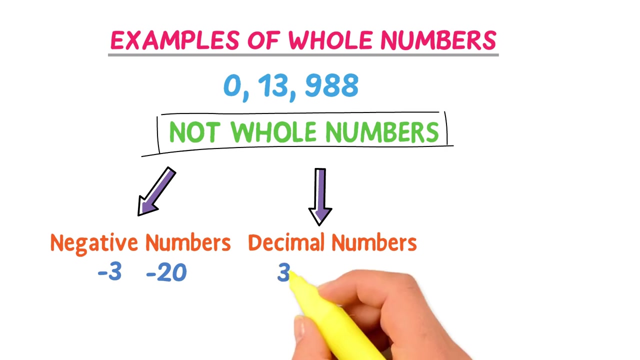 also a whole number. No, what are not whole numbers? Well, all the negative numbers are not whole numbers, like minus 3,, minus 20, etc. Secondly, all the decimal numbers are not whole numbers, like 3.6, 8.9, etc. Thirdly, all the 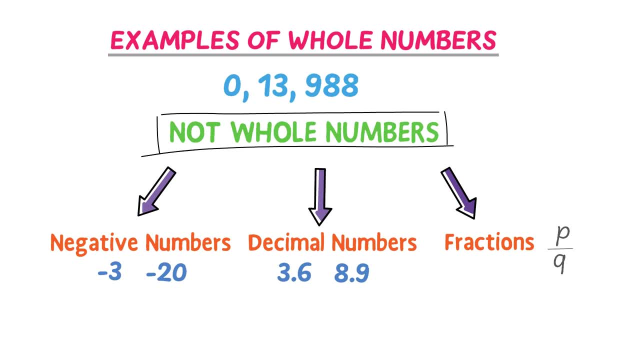 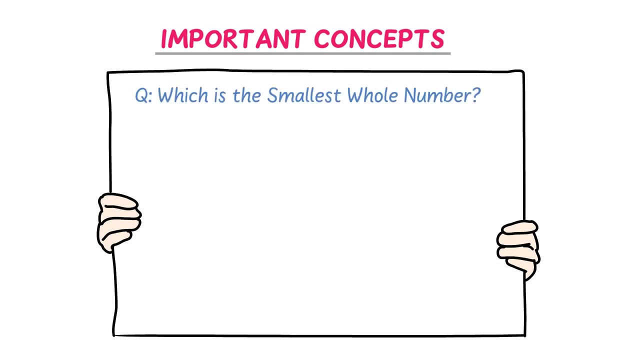 numbers in friction or p by q form are not whole numbers, like 2 upon 3,, 1 upon 6, etc. Finally, let me teach you some important concepts of whole numbers, like: which is the smallest whole number? Well, 0 is the smallest whole number There is. 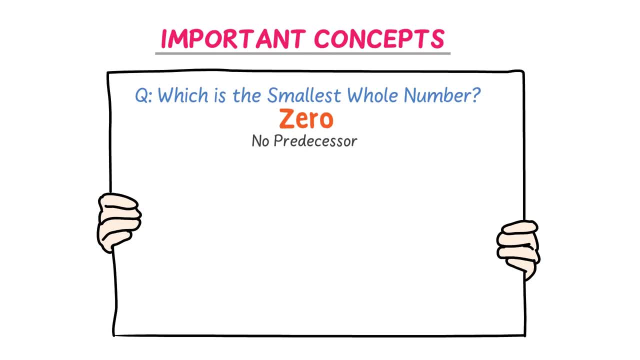 no predecessor or a number that comes before 0.. Let me repeat this important statement: There is no predecessor or a number that comes before 0.. Secondly, which is the largest whole number? Remember that there is no largest whole number, or we can say: 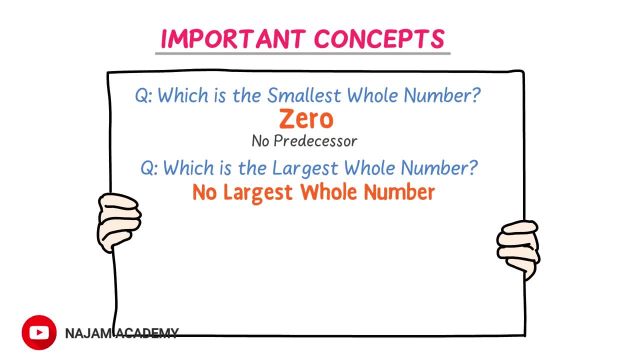 that no number is considered to be the largest whole number. Thirdly, can whole numbers be negative? Well, the answer is no. Whole numbers cannot be negative. Fourthly, can natural numbers be considered as whole numbers? The answer is yes, All the natural numbers are also considered as whole numbers. but 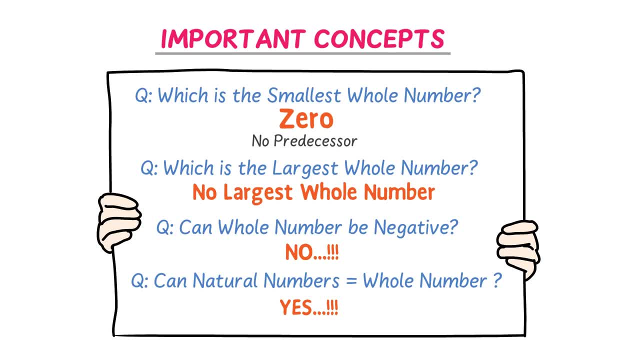 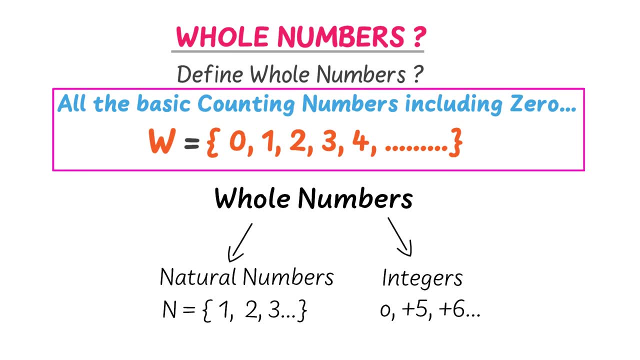 not all the whole numbers are considered as the natural numbers. To summarize my lecture, we learn that all basic counting numbers are whole numbers, like 0,, 1,, 2,, 3, and so on, And the set of whole numbers is denoted by w. Secondly, we learn that all 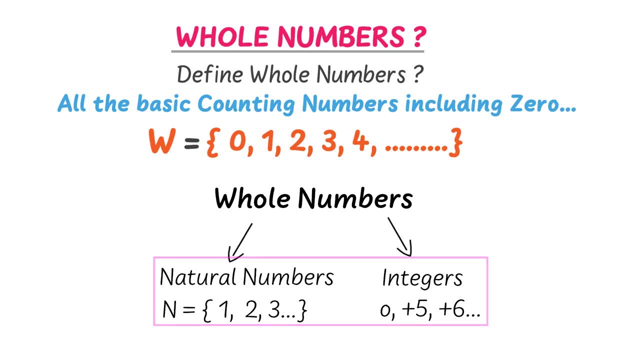 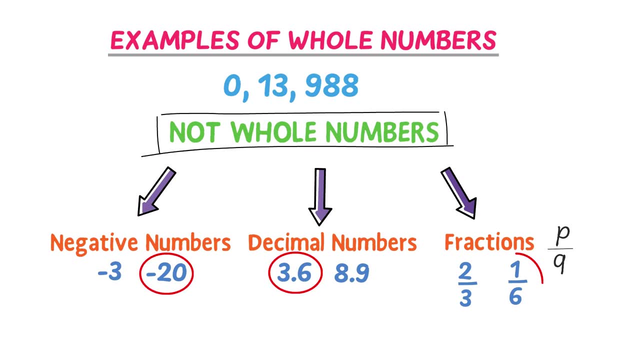 natural numbers and positive integers are not whole numbers. So we learn that all natural numbers and positive integers are also whole numbers. Thirdly, we learn that numbers like minus 20, 3.6, and 1 upon 6 are not whole numbers. Finally, we learn that 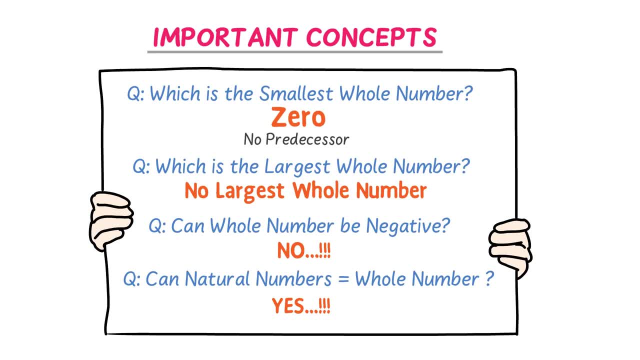 0 is the smallest whole number and there is no largest whole numbers. This was all about whole numbers.